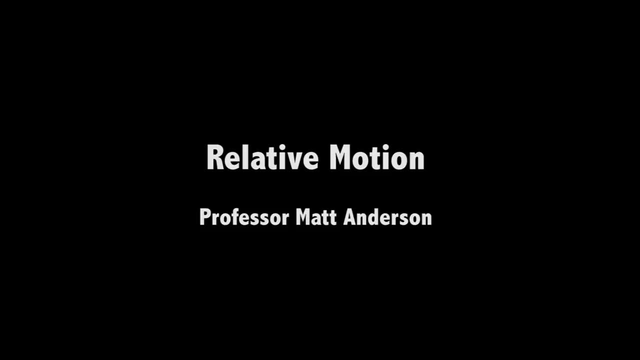 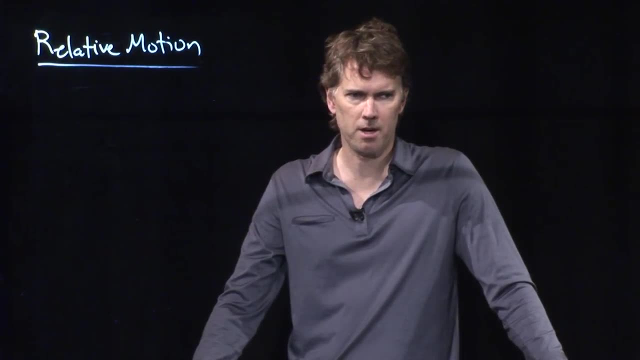 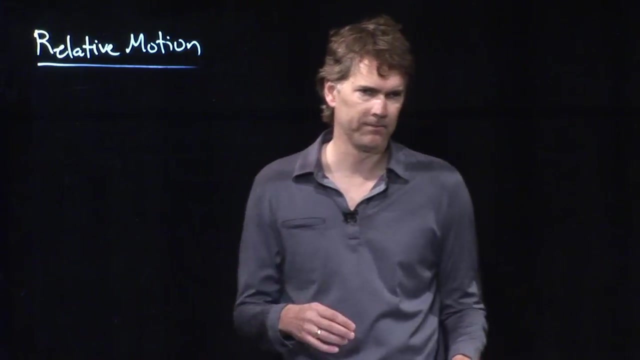 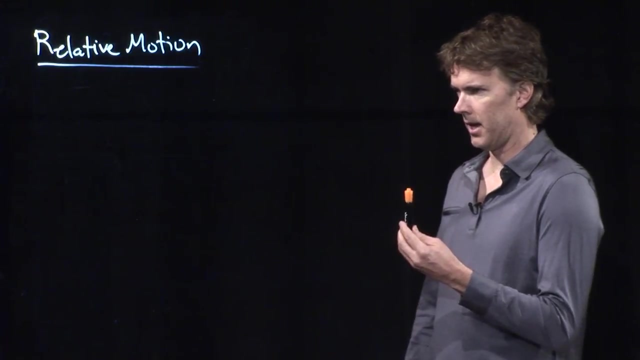 Hello class Professor Anderson. here Let's talk about relative motion. This is a very important concept in physics and it's this idea that motion is all really relative. So let's say we do the following experiment. I have a pen in my hand here and as I walk, 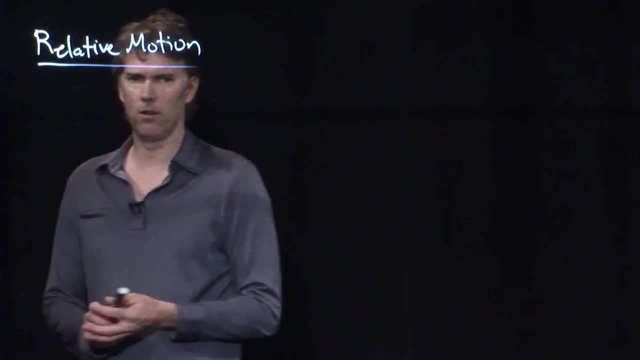 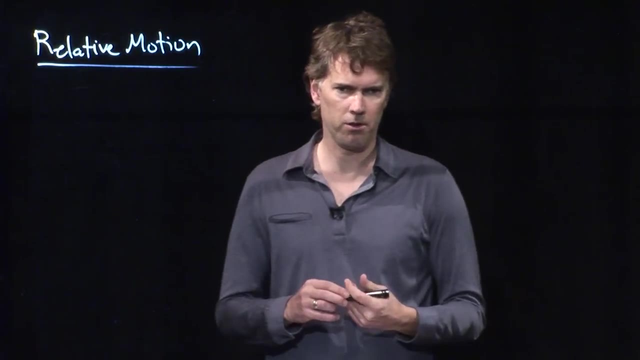 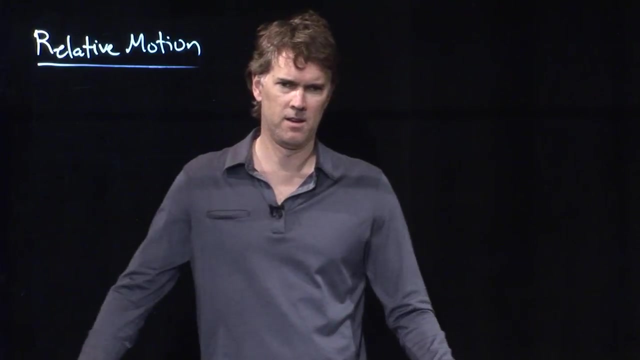 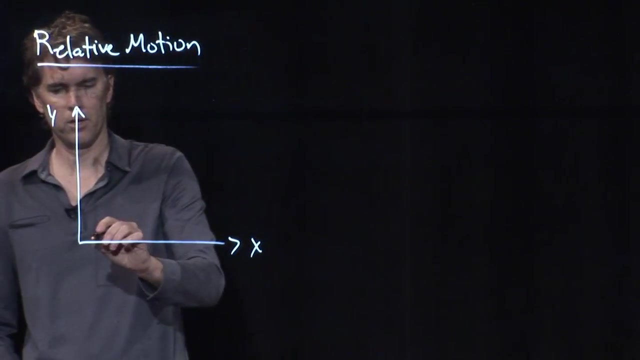 across the screen and I toss that pen straight up and down. what do you guys see in the audience? Somebody have a thought. Let me know. What do you think? What's the curve that you observe? Yes, Laura, A parabola, A parabola right Parabolic motion. So it would look something. 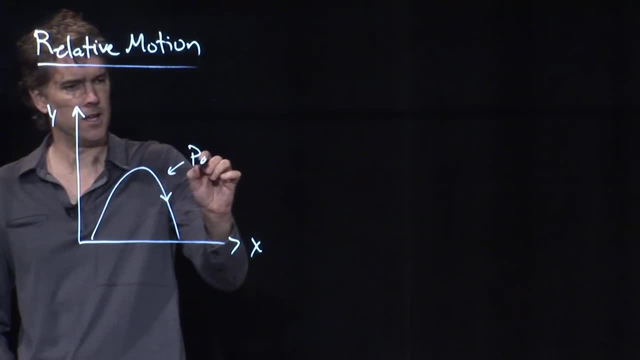 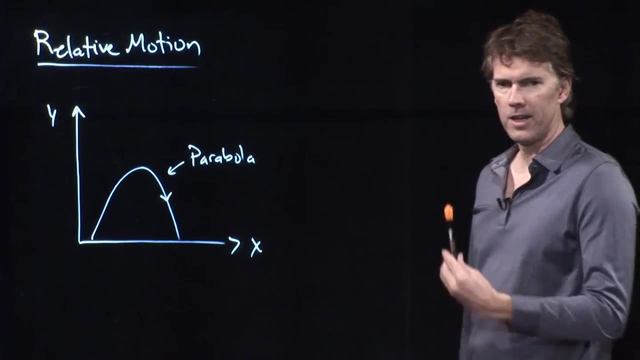 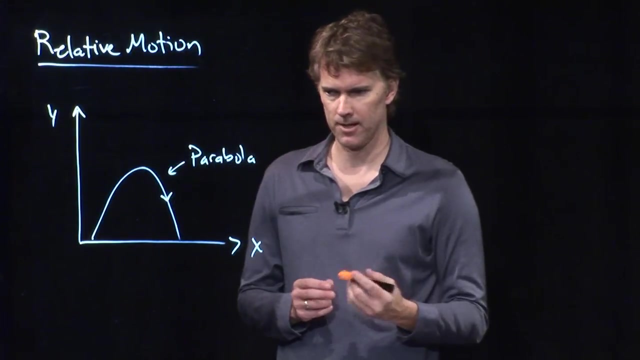 like that. Like you said, it is a parabola, And once that object leaves my hand, it is, of course, in free fall. The only thing acting on it is gravity, and we know that projectile motion maps out a parabola. But this is what you observed. 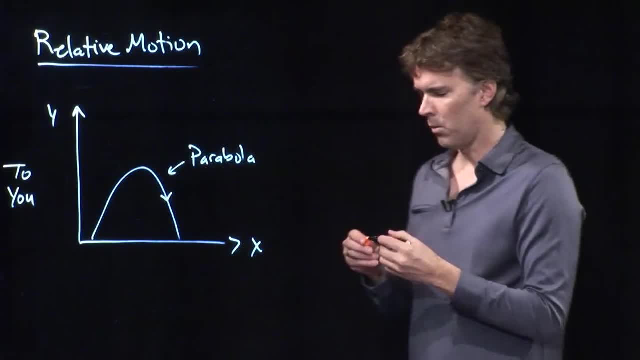 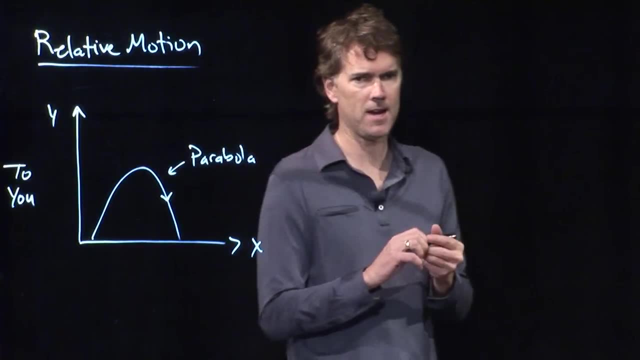 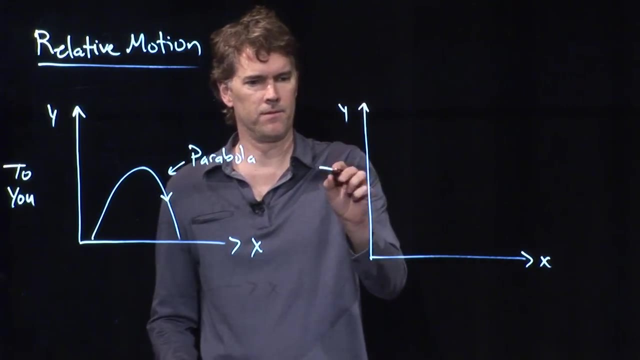 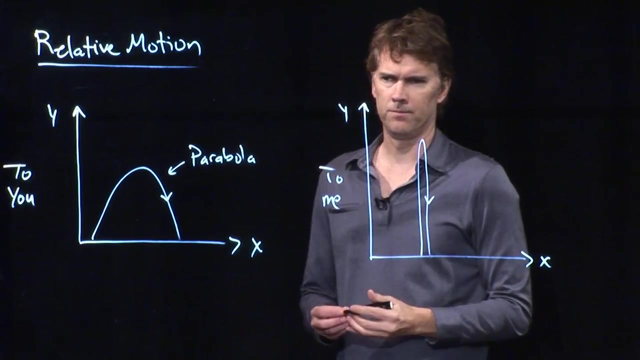 This is what it looks like to you, But what does it look like to me? right, As I walk across and I throw that object straight up and straight down, what I see is something very different To me. it looks like that thing went straight up and straight down. My coordinate system was: 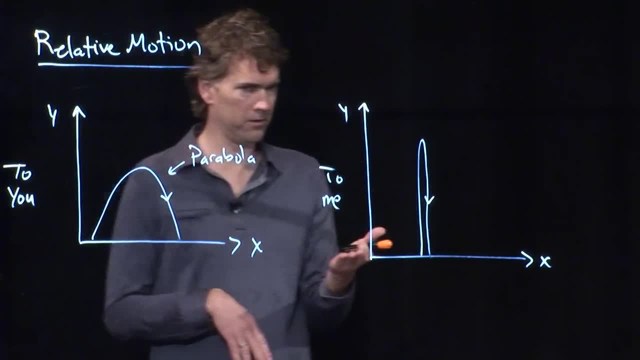 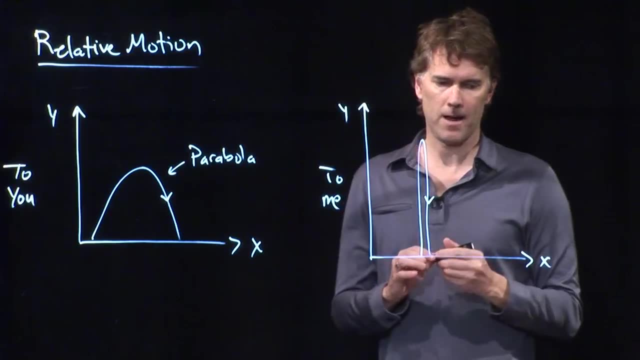 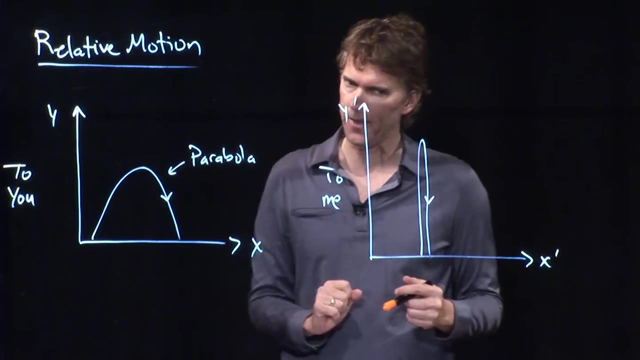 moving with me. Your coordinate system was stationary in the lab frame, And so those are two different coordinate systems And in fact, what we should do is probably call this the x prime- y prime frame, to denote that it's different than the x- y frame, And so this idea of relative. 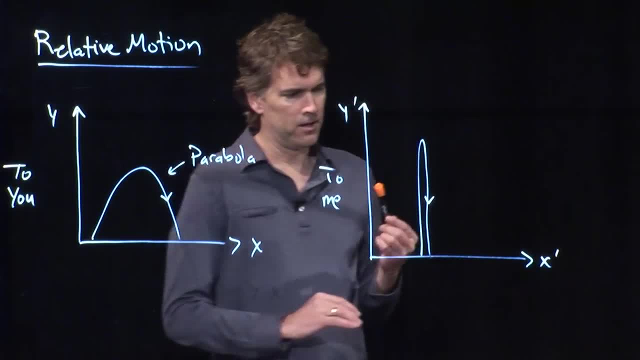 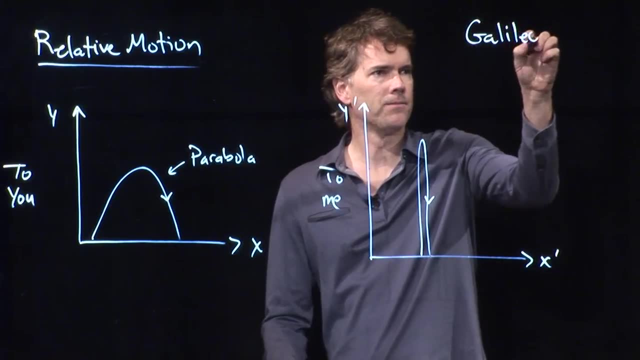 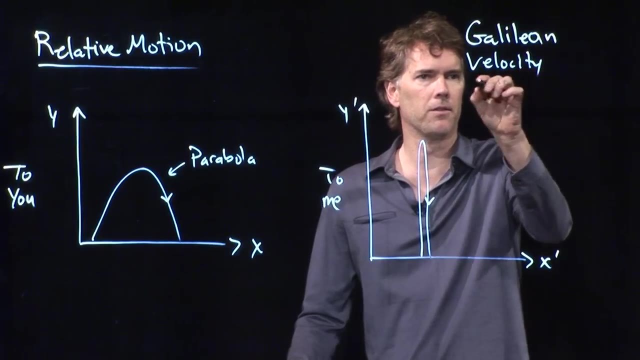 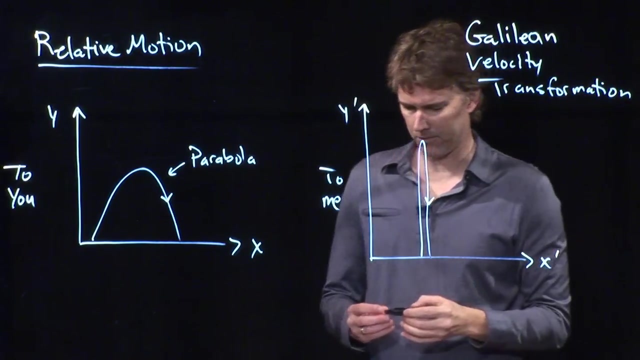 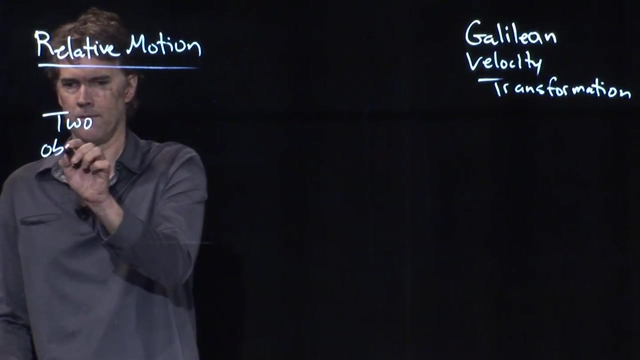 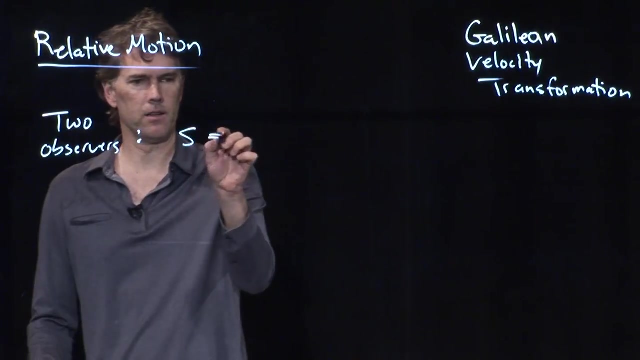 motion is really important, And the person that came up with the idea originally was Galileo, And he wrote down something called the Galilean Velocity Transformation And we're going to see how that works. Okay, let's say we have two different observers That could be like me and you, And s is the stationary. 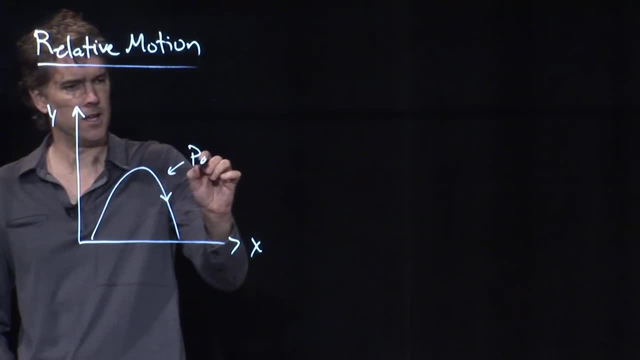 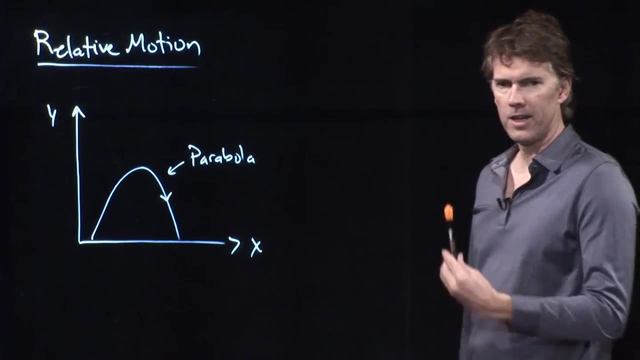 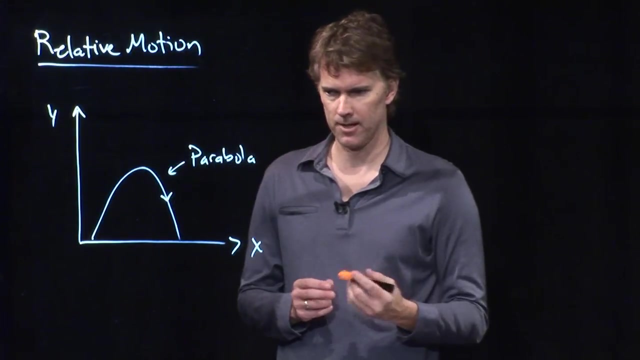 like that. Like you said, it is a parabola, And once that object leaves my hand, it is, of course, in free fall. The only thing acting on it is gravity, and we know that projectile motion maps out a parabola. But this is what you observed. 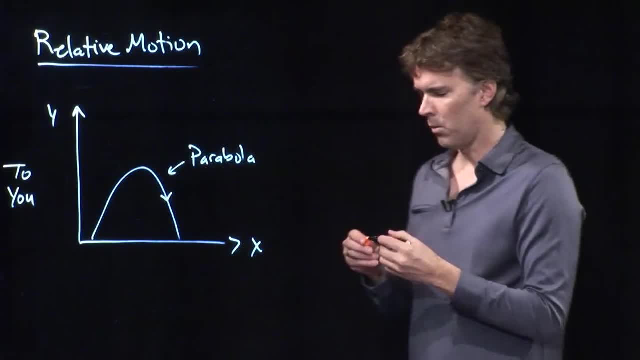 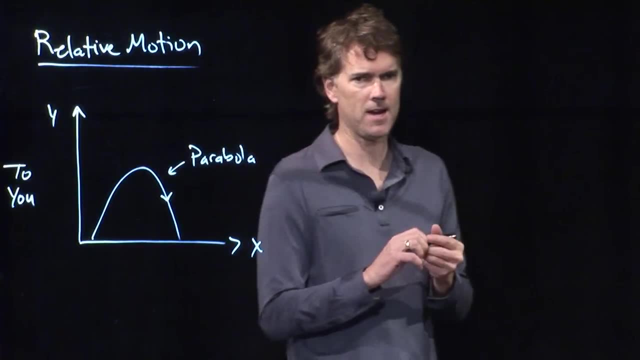 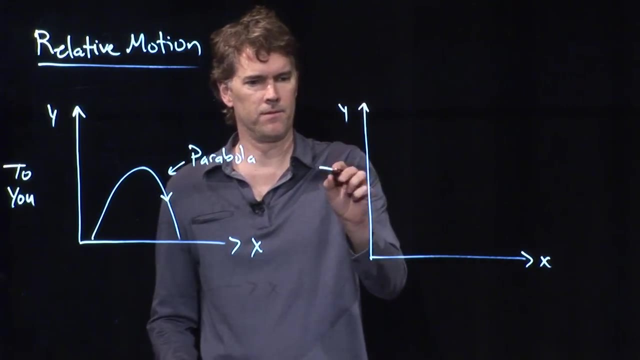 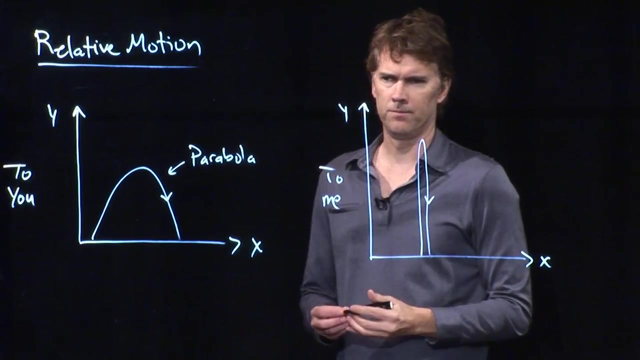 This is what it looks like to you, But what does it look like to me? right, As I walk across and I throw that object straight up and straight down, what I see is something very different To me. it looks like that thing went straight up and straight down. My coordinate system was: 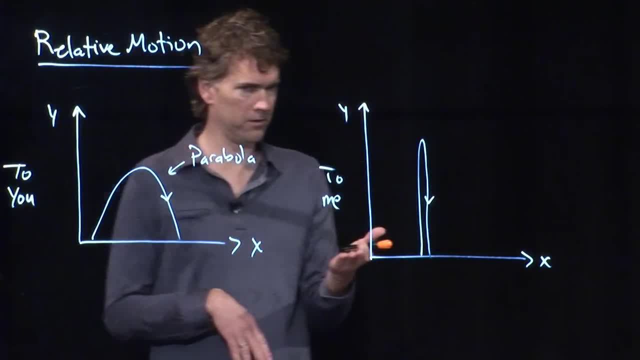 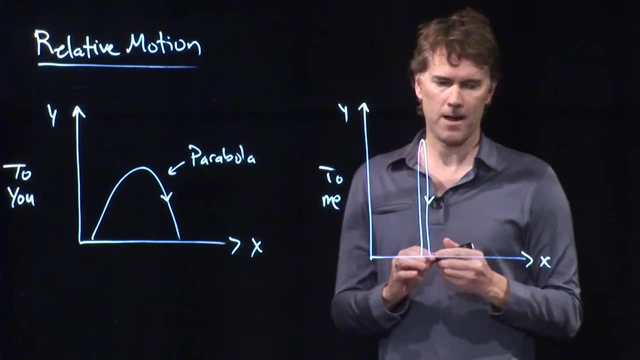 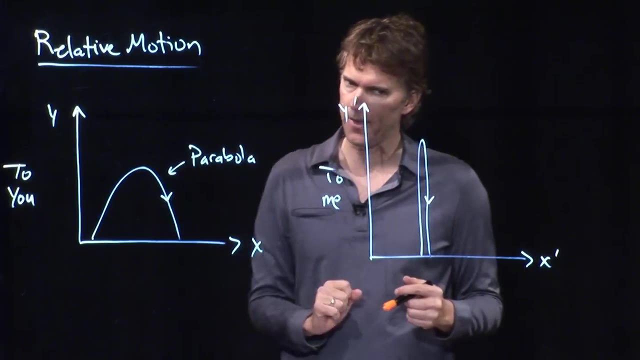 moving with me. Your coordinate system was stationary in the lab frame, And so those are two different coordinate systems, And, in fact, what we should do is probably call this the x prime, y prime frame, to denote that it's different than the x-y frame, And so this idea of 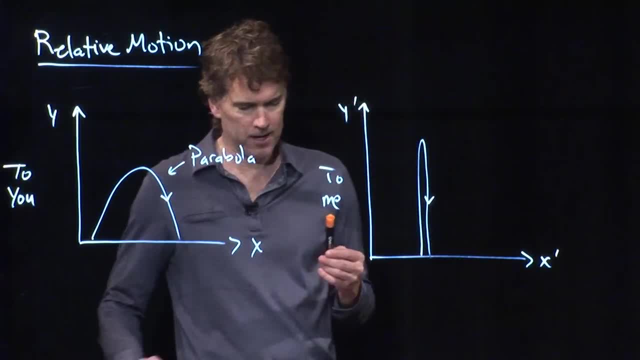 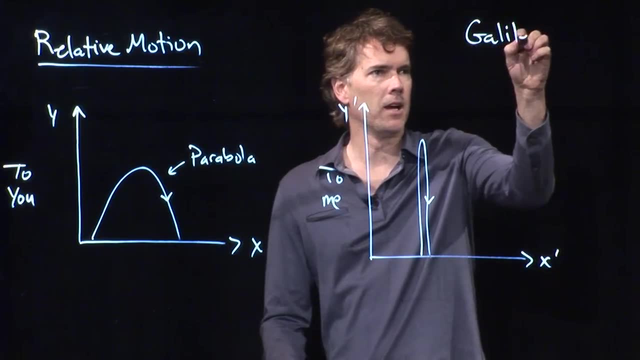 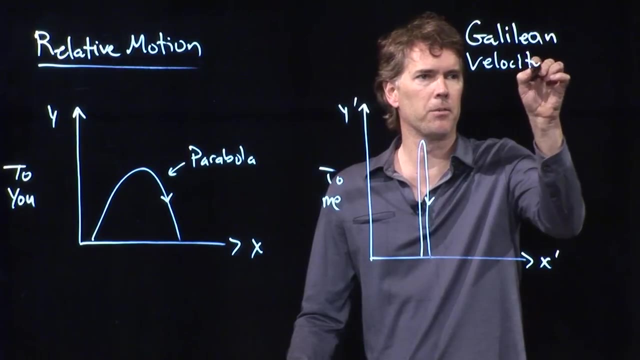 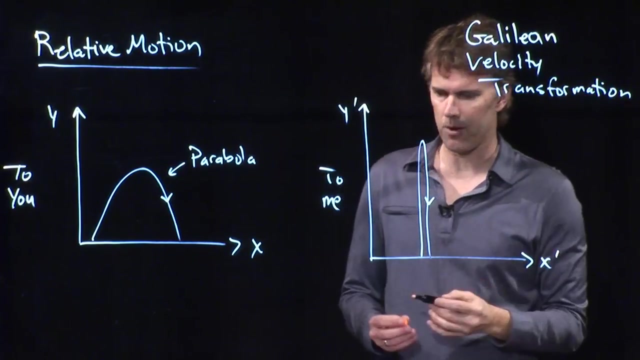 relative motion is really important, And the person that came up with the idea originally was Galileo, and he wrote down something called the Galilean velocity transformation And we're going to see how that works. Okay, let's say we have two different observers. 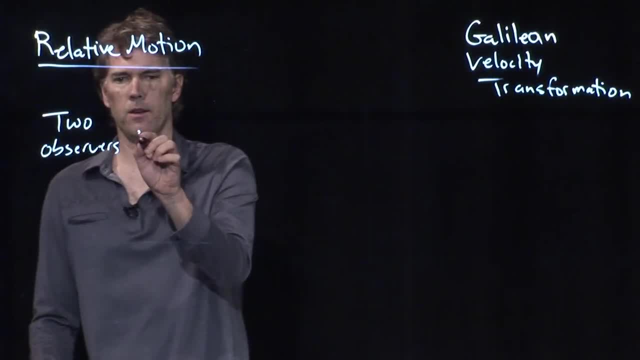 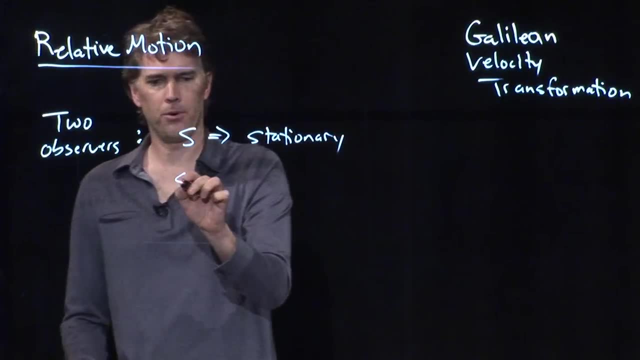 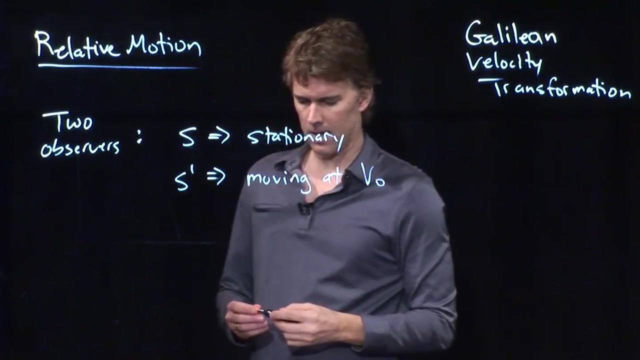 That could be like me and you And S is the stationary observer, That's you S prime is the moving observer, That's me, okay, and I am moving at a speed V naught, All right. how can we make sense? 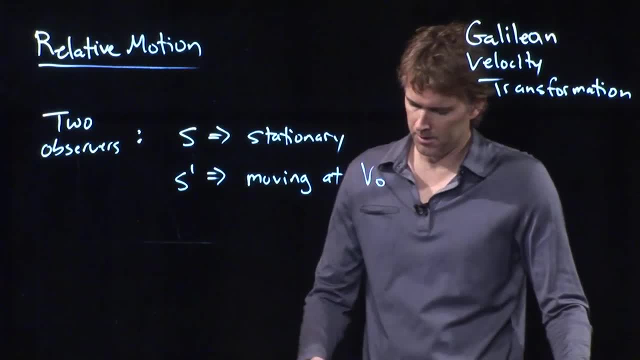 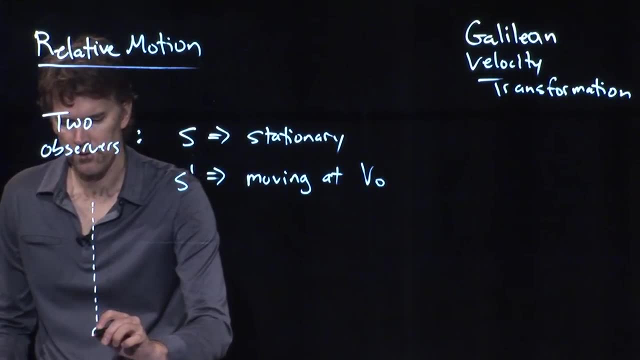 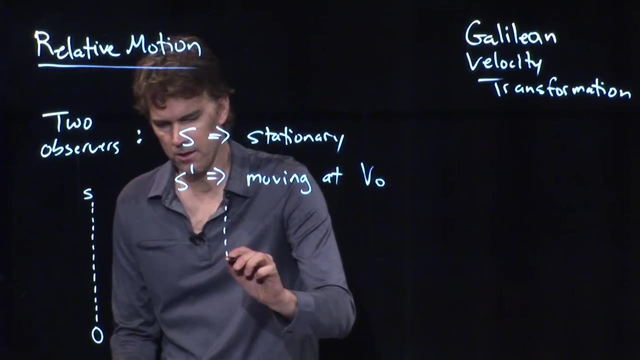 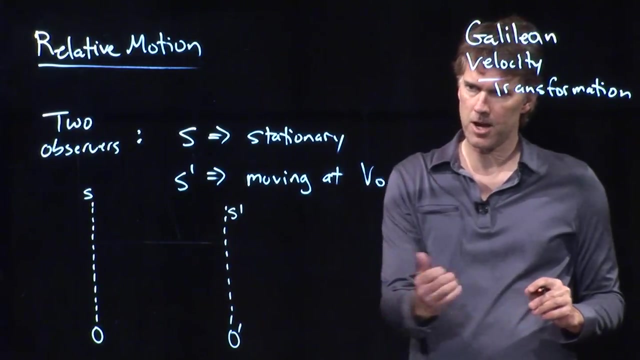 of what you observed versus what I observed. Well, the way we do it is the following: Let's draw an origin for the S frame and let's draw a different origin for the S prime frame. All right, and we know that the S prime frame is moving along. 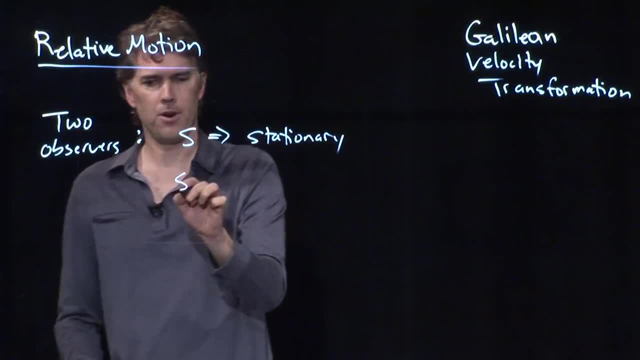 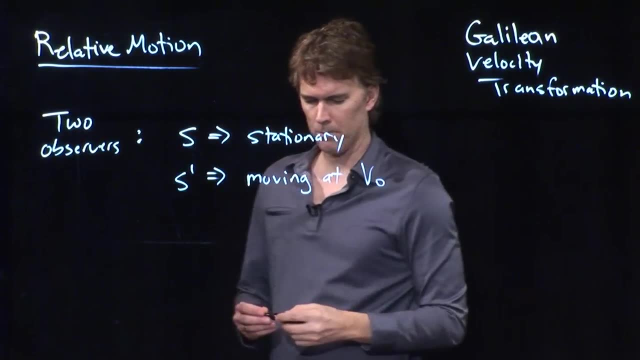 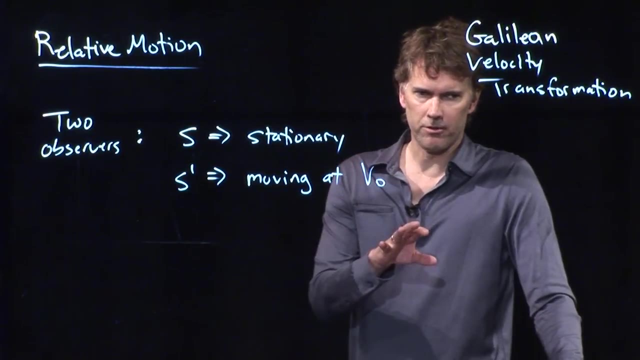 observer, That's you S prime, is the moving observer. That's me, Okay, and I am moving at a speed of v naught, Alright. how can we make sense of what you observed versus what I observed? Well, the way we do it is. 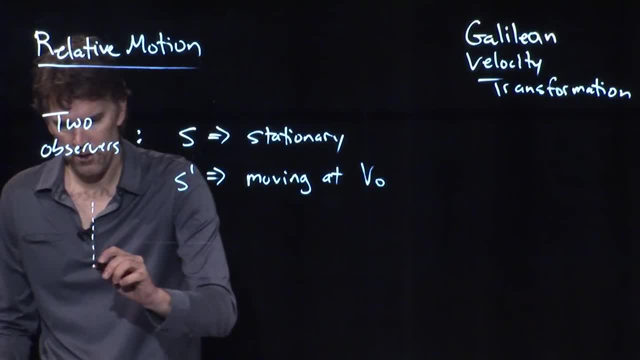 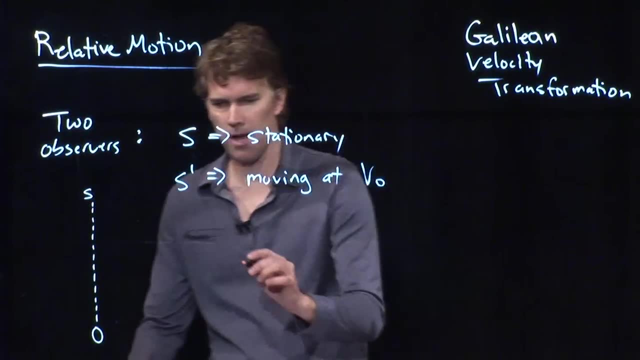 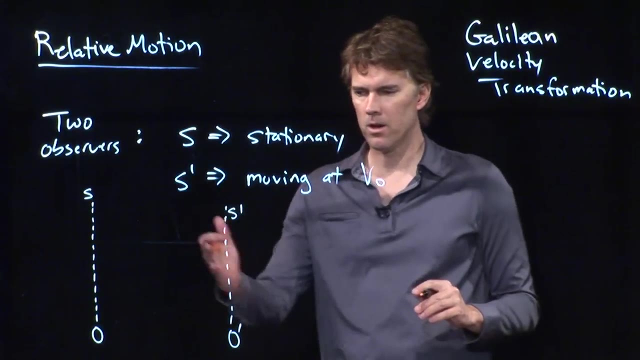 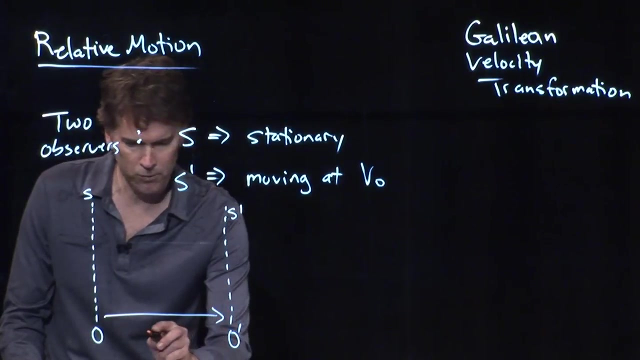 the following: Let's draw an origin for the s frame And let's draw a different origin for the s prime frame. And we know that the s prime frame is moving along relative to the s frame, And it's in fact moving at speed. v naught. 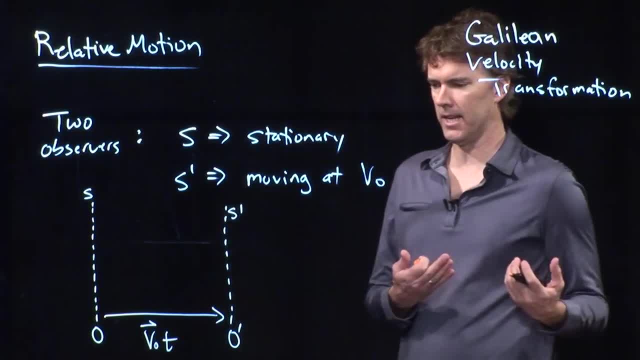 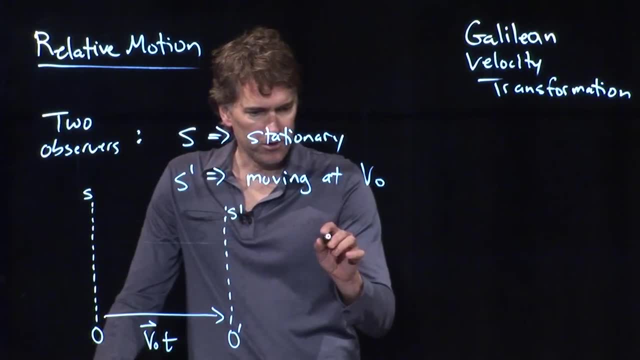 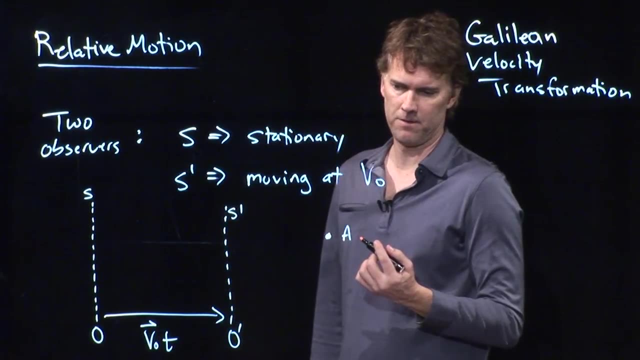 So in a time t it will traverse a distance v naught t. Okay, just increases as a function of time. Now, something that we observe is sitting up there at a. That could be the position of the pen when I tossed it. 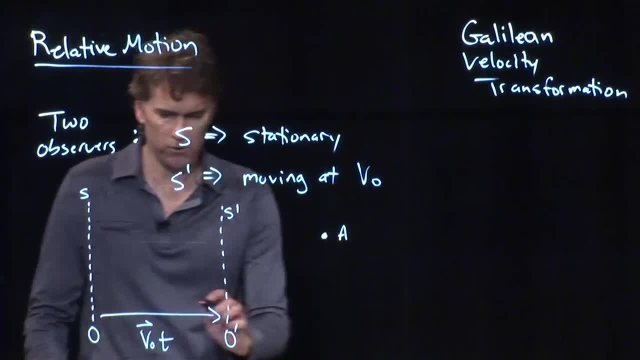 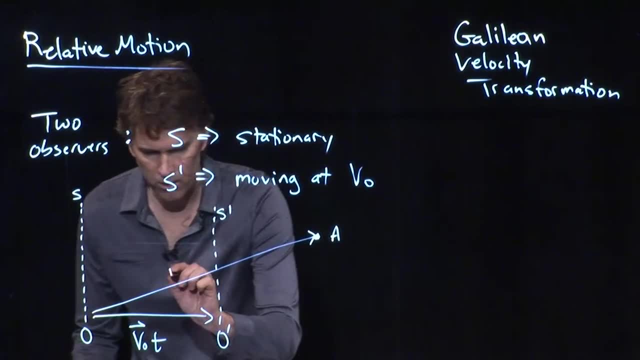 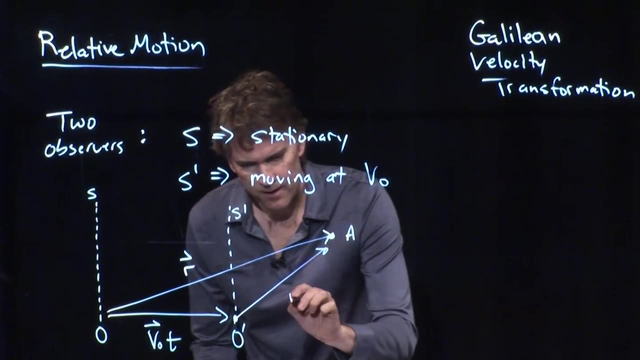 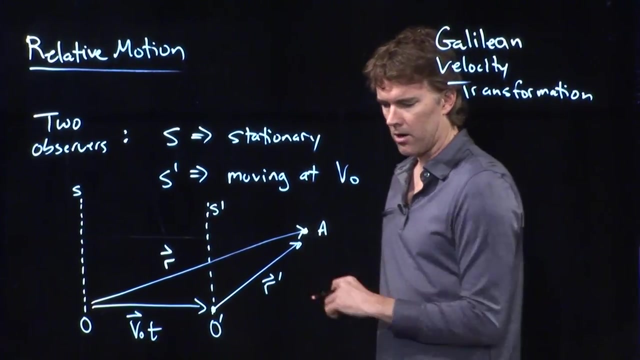 O to a is what you observe, That is the position vector that you observe, And we can call that r. But O prime to a is what the moving observer observes And that we can call r prime. Alright, so this maybe looks a little complicated. 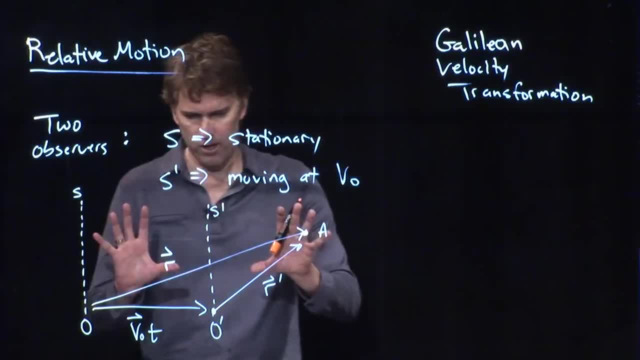 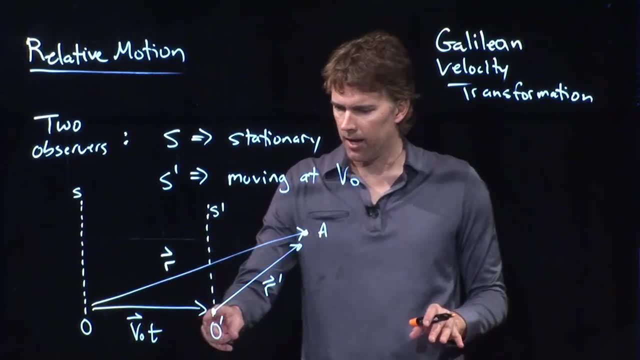 But we are familiar with vectors, right, We know how to add up vectors. It looks like if I take this vector v, naught t and I add r prime, I'm going to get the sum of the two, which is r. 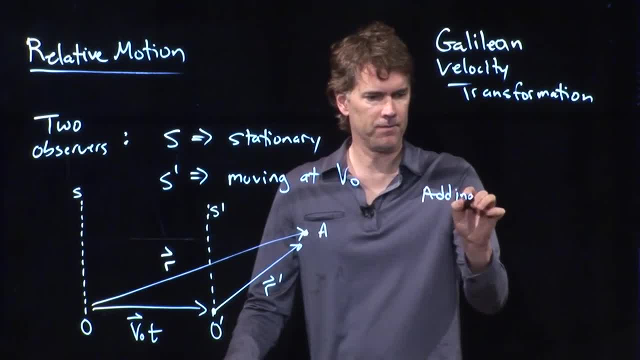 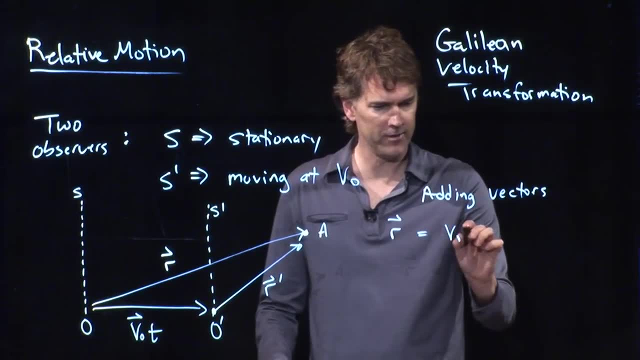 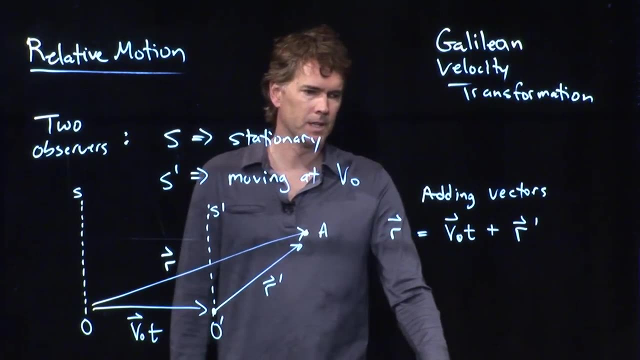 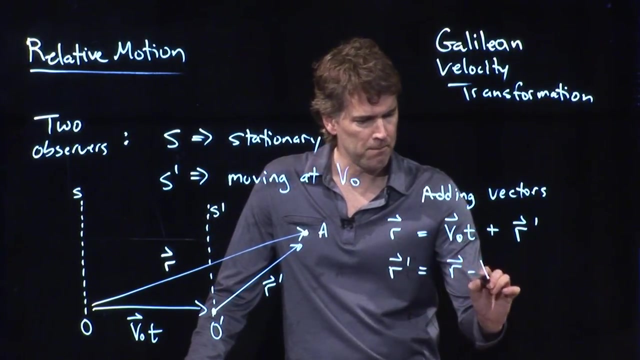 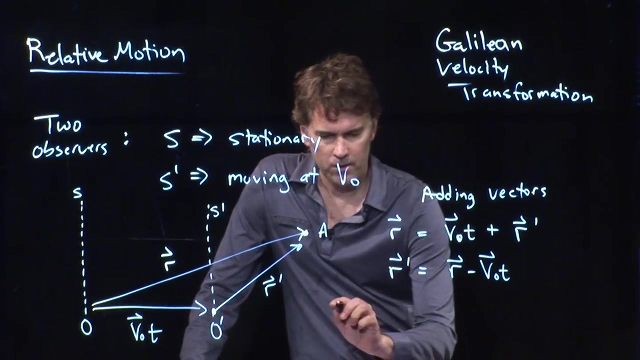 And that's exactly what we do. r is just the sum of v naught t plus r prime, And now you can rewrite this for r prime if you're interested. r prime equals r minus v naught t, And now you can solve for v right. 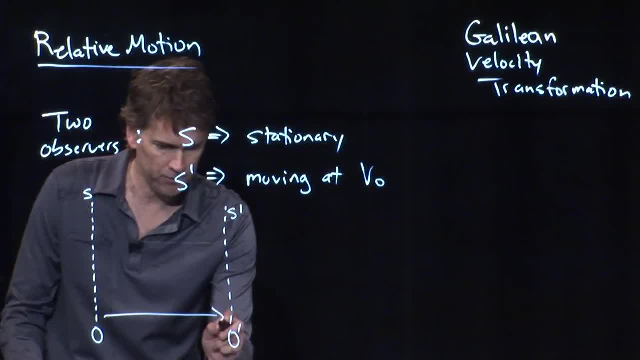 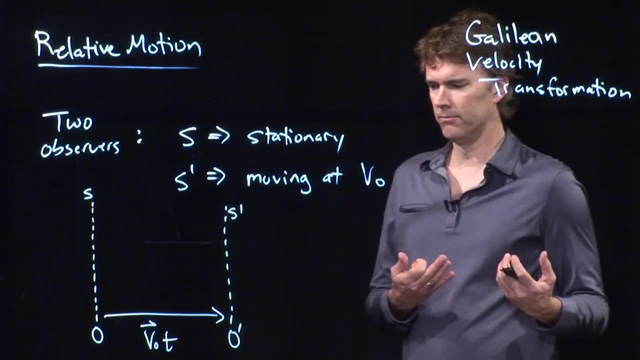 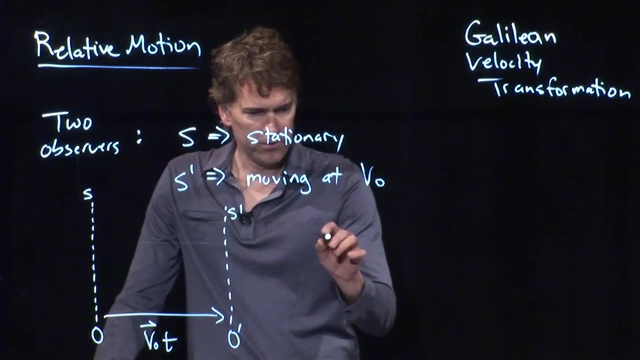 relative to the S frame, and it's in fact moving at speed V naught. so in a time T it will traverse a distance V naught. T Okay, just increases as a function of time. Now, something that we observe is sitting up there at A. 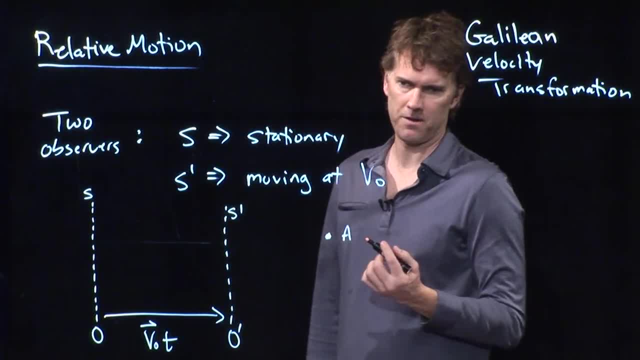 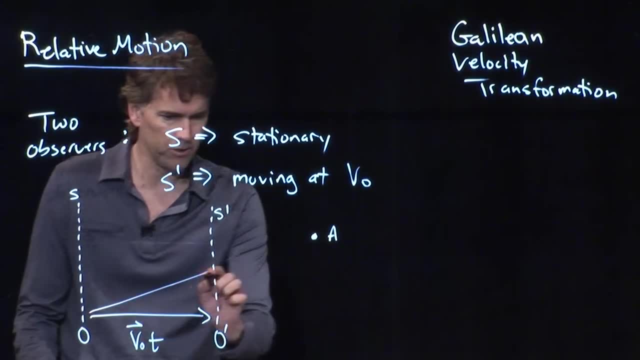 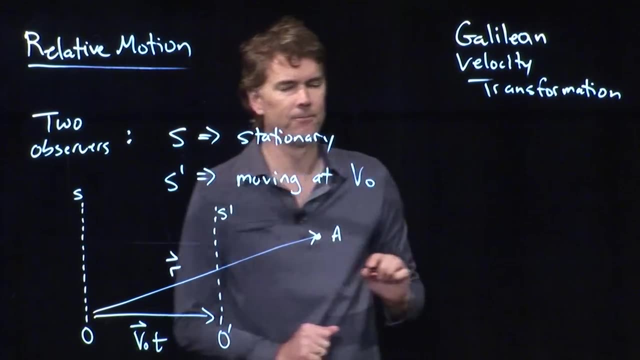 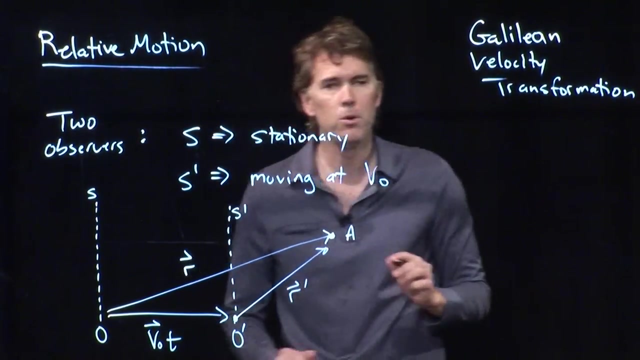 That could be the position of the pen when I tossed it. So O to A is what you observe, That is the position vector that you observe, and we can call that R, But O prime to A is what the moving observer observes. 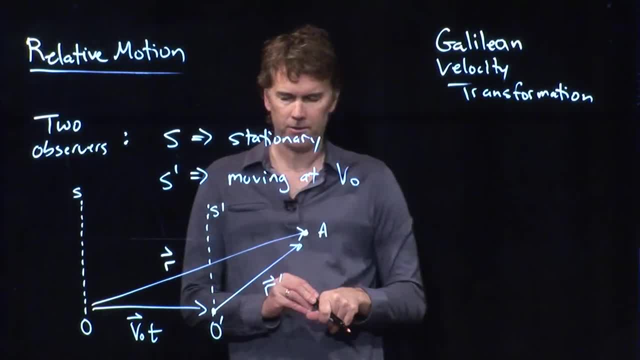 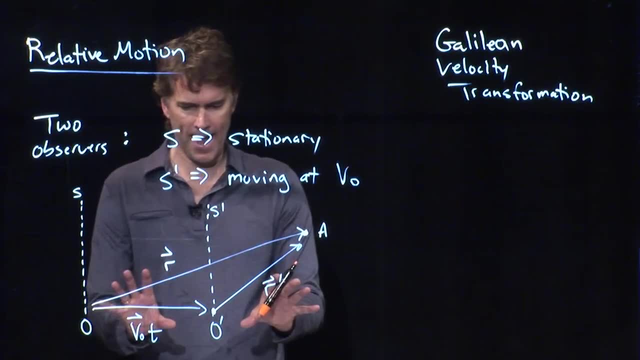 and that we can call R prime. All right, So this maybe looks a little bit weird, It's a little complicated, but we are familiar with vectors. right, We know how to add up vectors. It looks like if I take this vector V naught T and I add R prime. 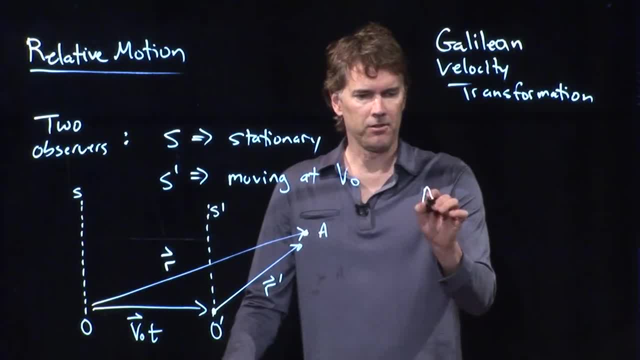 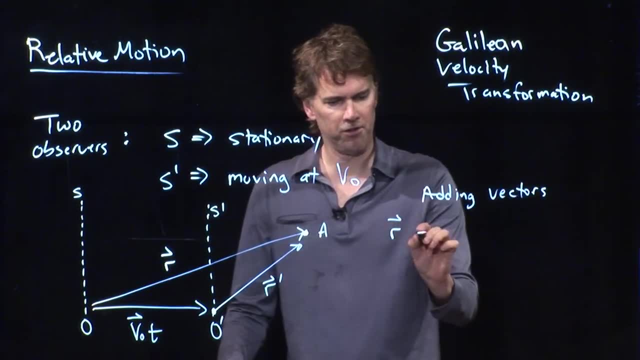 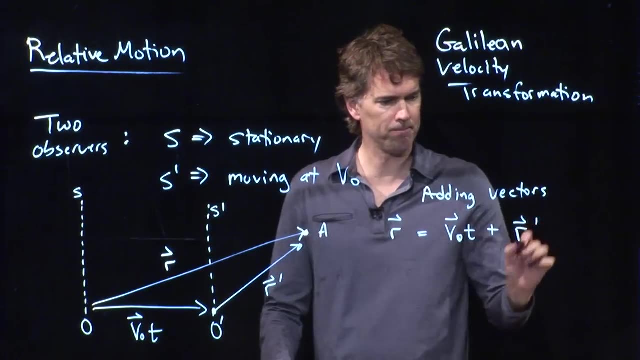 I'm going to get the sum of the two, which is R, and that's exactly what we did. R is just the sum of V, naught T plus R prime. Okay, And now you can rewrite this for R prime if you're interested. 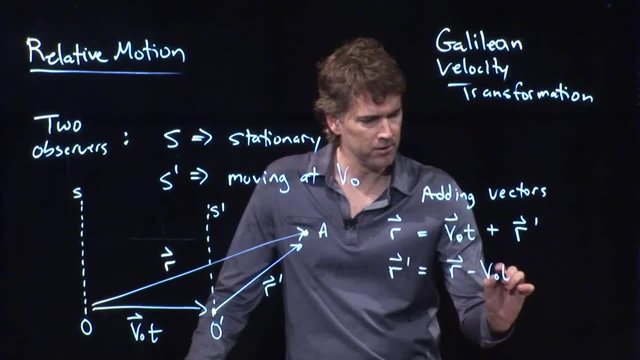 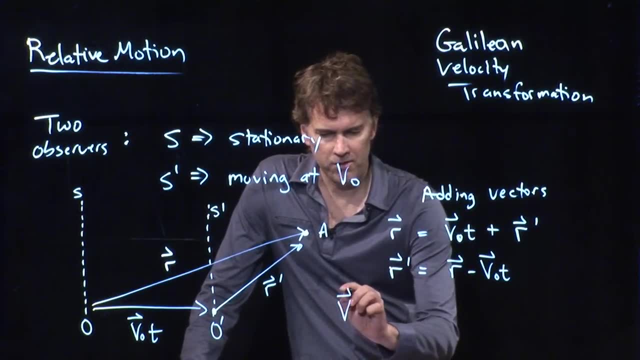 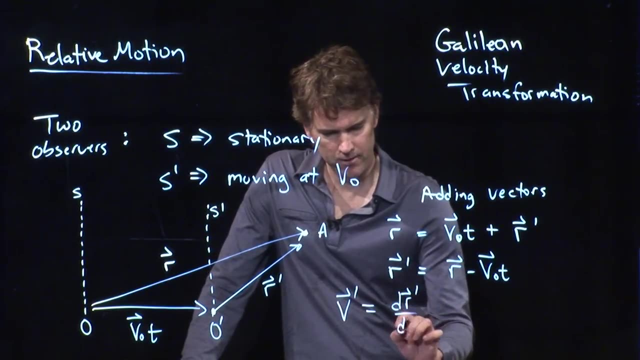 R prime equals R minus V, naught T, And now you can solve for V Right. What is the velocity observed in the moving frame? It's just the derivative of R prime with respect to T, And so I need to take a derivative of this thing. 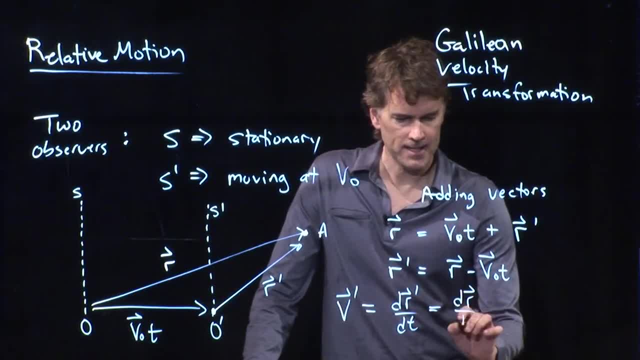 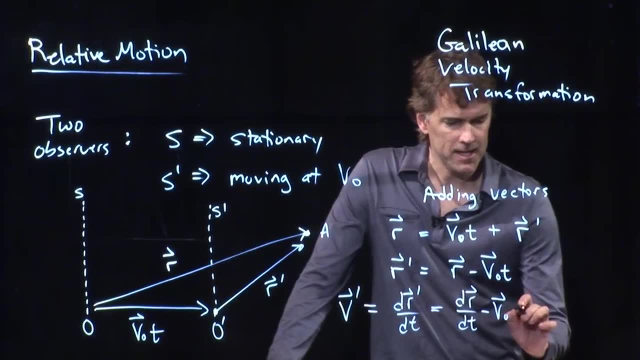 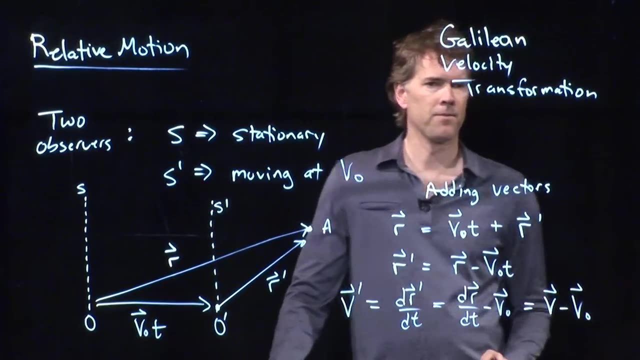 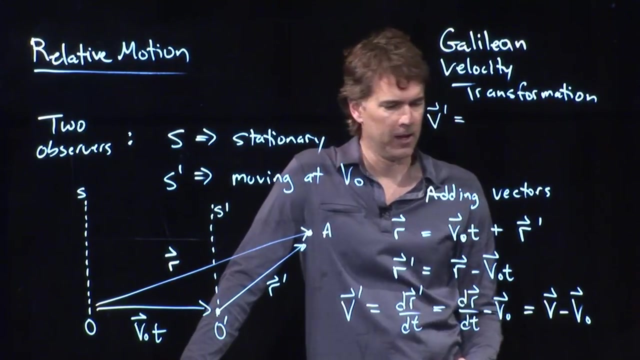 What do I get? I get dr dT minus V naught. So brdT is just the speed observed in the stationary frame, And so this is the Galilean velocity transformation. What is the velocity observed in the moving frame? It is the velocity observed in the stationary frame minus the 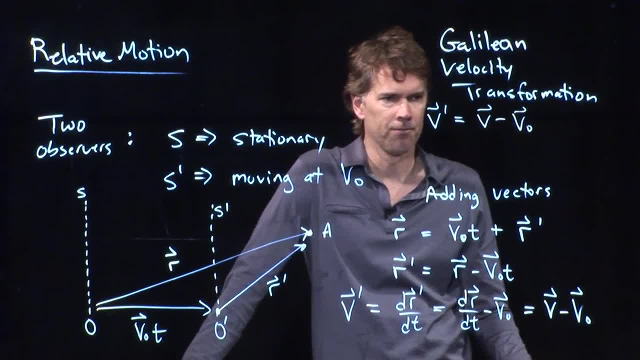 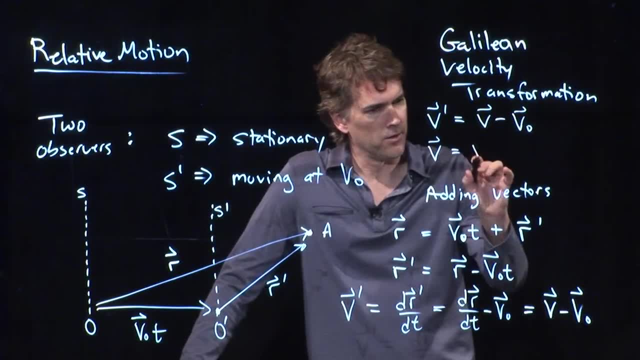 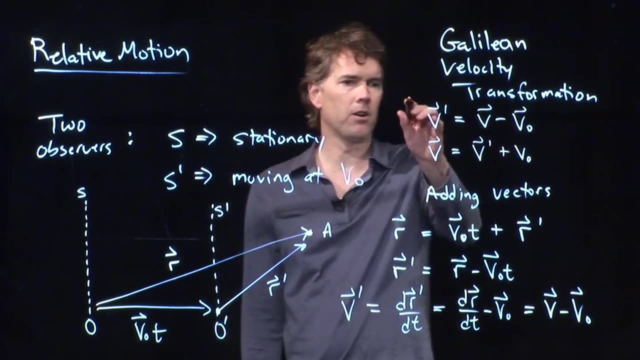 velocity observed in the investments plus the velocity of the moving frame. You can, of course, rewrite this: the velocity in the stationary frame is going to be the velocity in the moving frame plus that. Okay, so these are known as the Galilean velocity transformations. 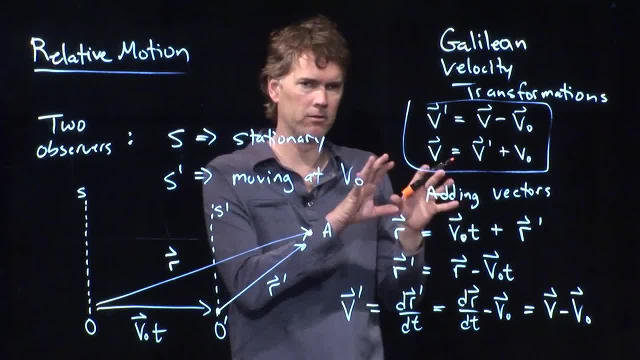 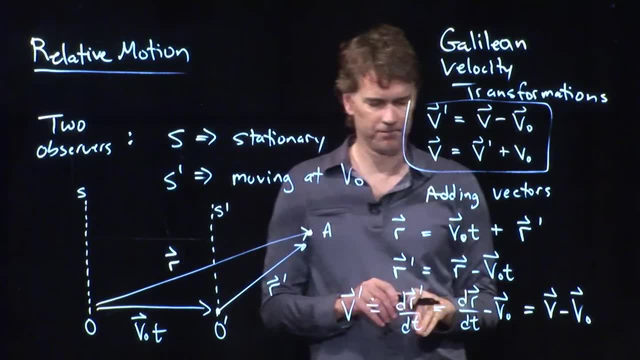 And it should make sense to you, right? You just add or subtract velocities, but you have to treat them as vectors. Let's try an example of this. 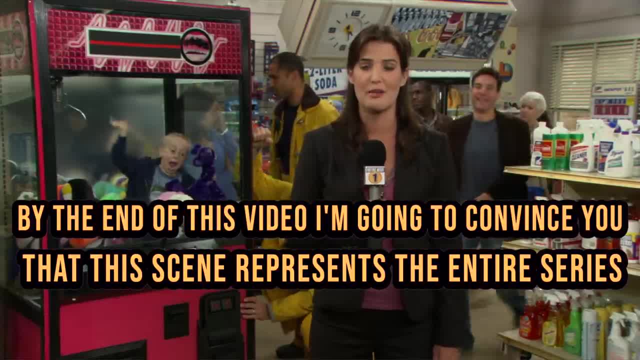 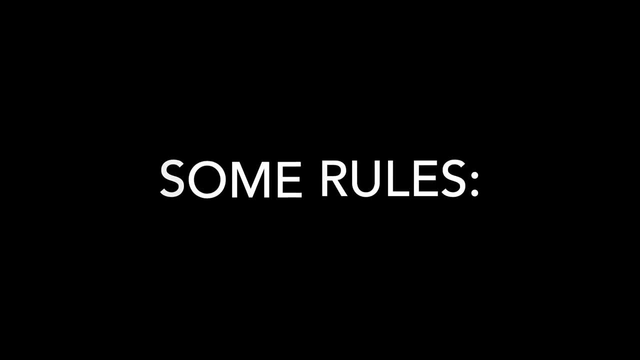 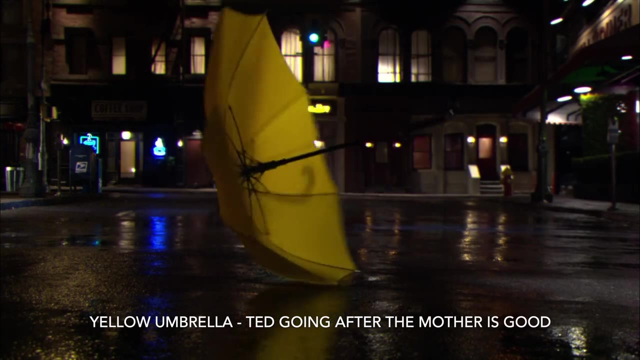 All in the pursuit of a stuffed purple giraffe From Metro News 1,. I'm Robin Trevatsky, We're clear. Thanks, Don. You know the short version, the thing with your mom's yellow umbrella. But there's a bigger story. 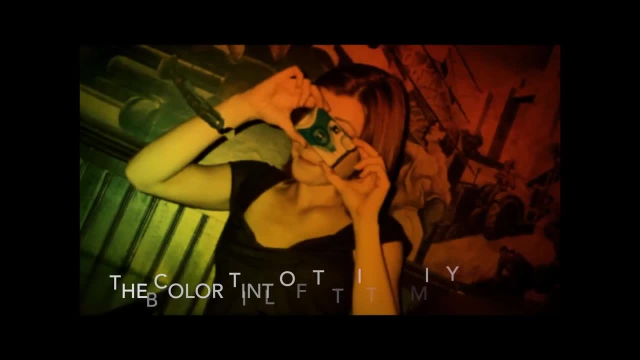 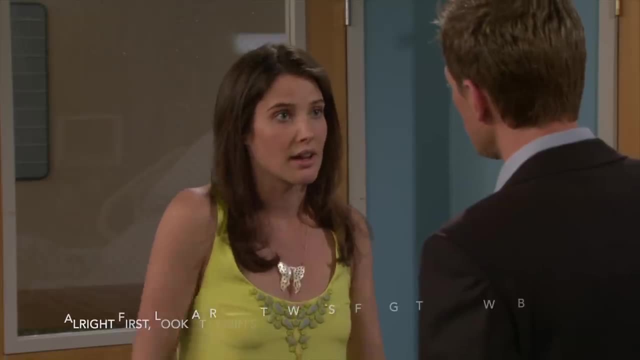 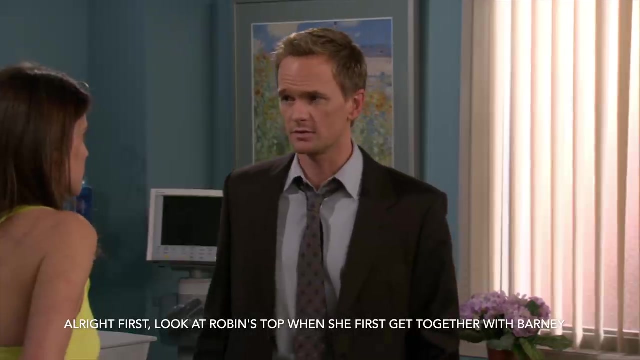 The story of how I became who I had to become before I could meet her. It's not your thing. I thought I'd save you the trouble. Maybe I don't want to be saved the trouble. Maybe I want the trouble. I haven't wanted the trouble in a long time. 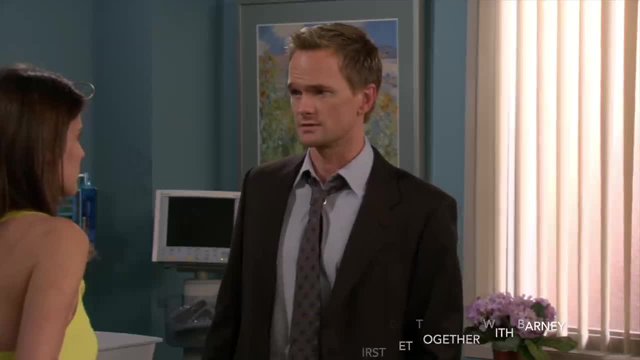 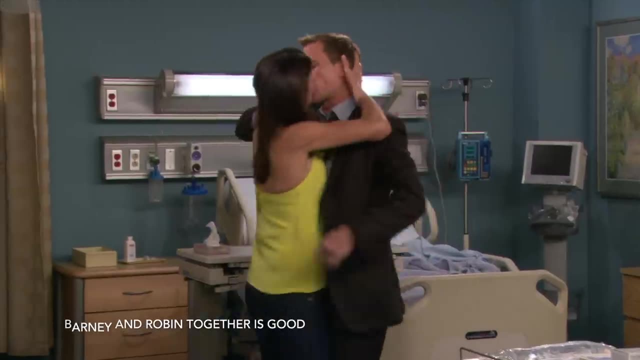 But with you the trouble doesn't seem so troubling. Okay, friends, then I love you, Let's get married. No, you're smothering me. Okay, forget it. Gah Coming out of retirement For one last time. 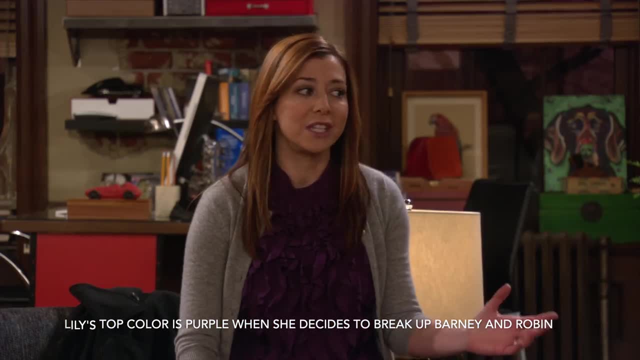 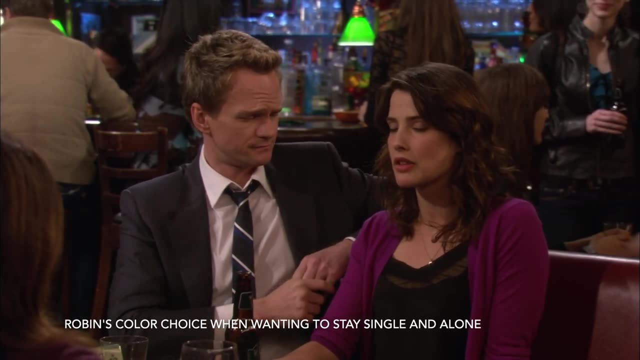 Let's break up. Whoa, Yes, All right. how are we gonna do it? These guys are in so deep. just one fight ain't gonna do it. Enchanté, That's French for what's with the purple. Well, tomorrow's Valentine's Day and everything is pink and red. 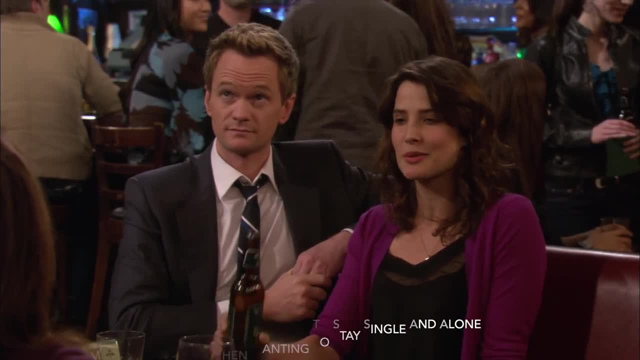 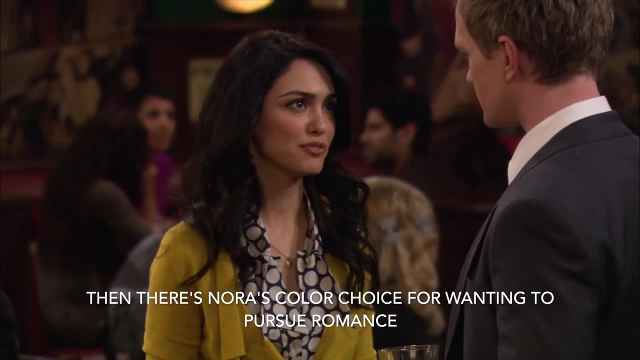 So Bev very thoughtfully suggested that we wear purple to show how little we care. Hey, hey, sorry, Oh hi. Quick question: Yeah, Why aren't you wearing purple like your friends? Oh, I told them I forgot, but the truth is I'm kind of protesting their protest. 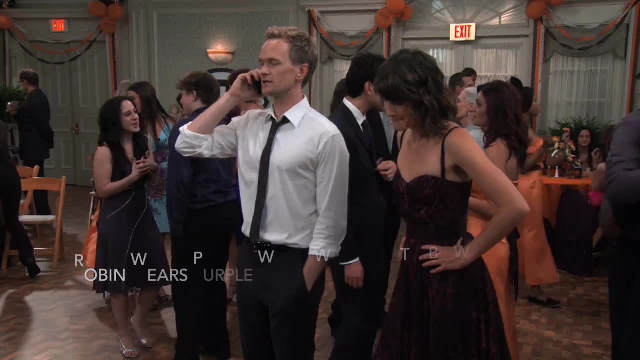 Can you keep a secret? Sure, I love Valentine's Day. The reason that I called is, Uh, To tell you, To tell you how I feel about you. To tell you how I feel about you. I know we didn't work out the first time.